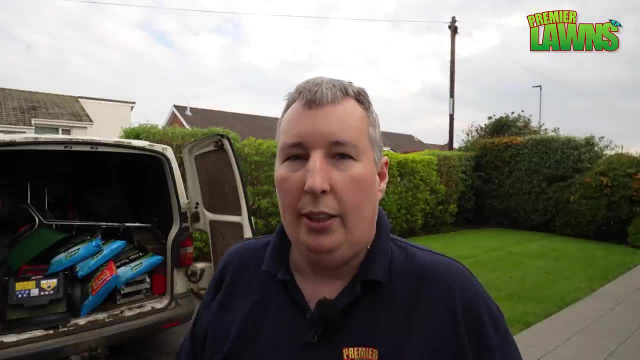 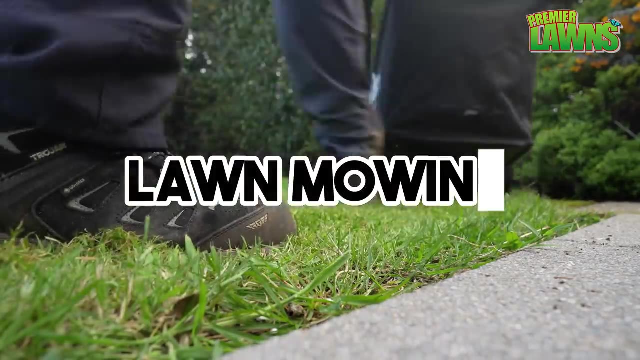 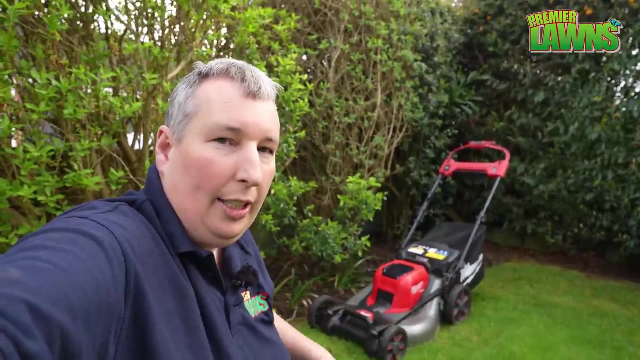 association with Milwaukee Tools UK. but more on that later. Let's go. The first task in any lawn renovation is to get the grass cut. That's what I'm going to be doing now. Now, in some of my lawn renovation videos, you see us: we don't cut the grass, but I'm trying to. 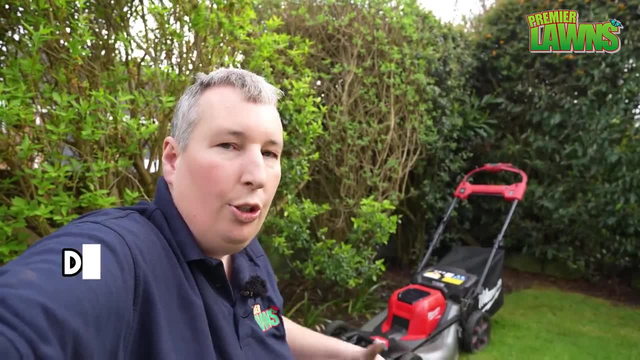 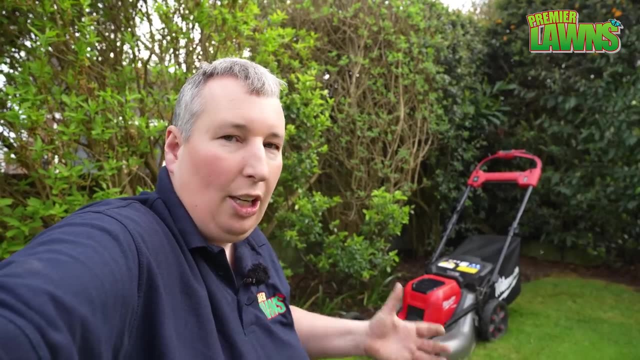 show you, if I was a homeowner, if this was my lawn, what I would do. Should you save the grass right down, or shouldn't you? Today, I'm going to cut the grass a bit shorter than usual, but I'm not going to save it right down. That comes down to personal preference. Now I'm going to show you. 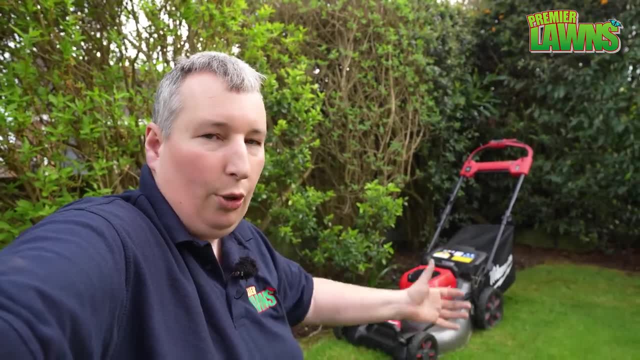 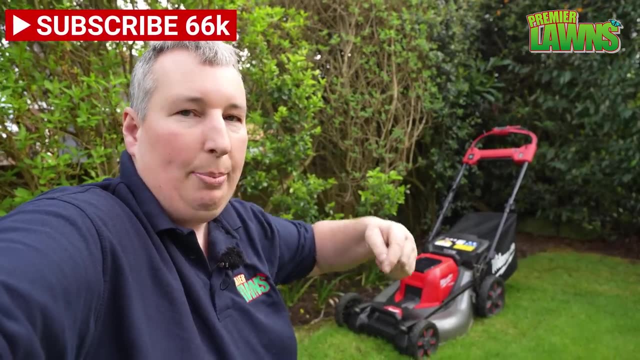 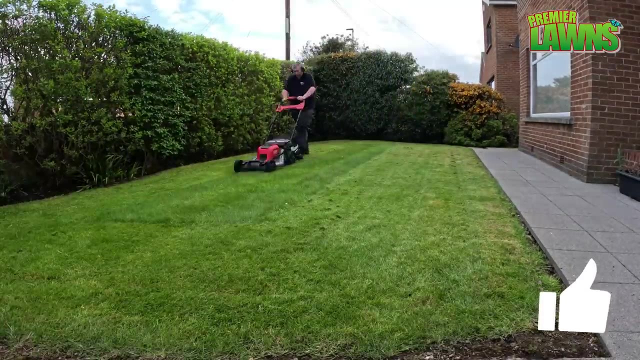 exactly how this lawn goes for the next few weeks. If you want updates on what this lawn looks like in a week, in two weeks or three weeks, make sure to subscribe and you can follow along the journey on my community page. We're going to have a look. You can see that there's a bit of thatch there. 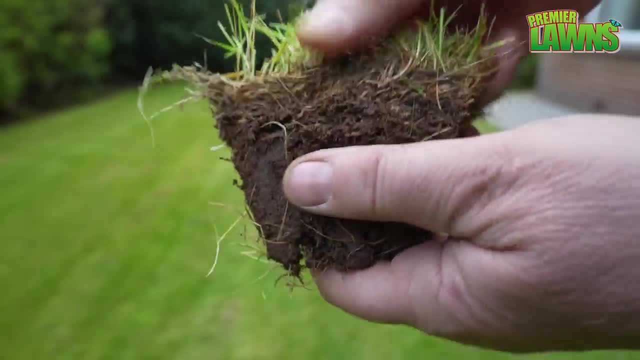 so we're going to see our soil and then we're going to see our thatch. So this layer of material here, Some thatch, is healthy, but if you have too much thatch then it becomes unhealthy and it doesn't have a good life. I've got grass here, so I'm going to be cutting it up for you. 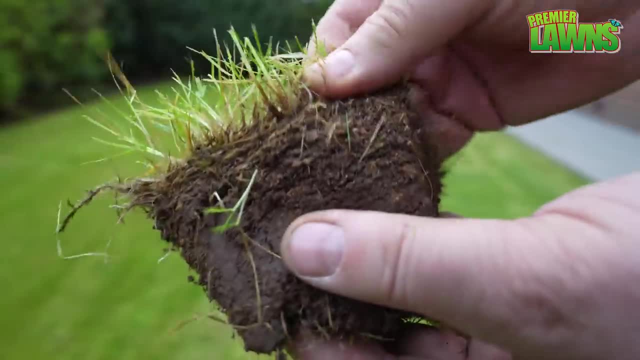 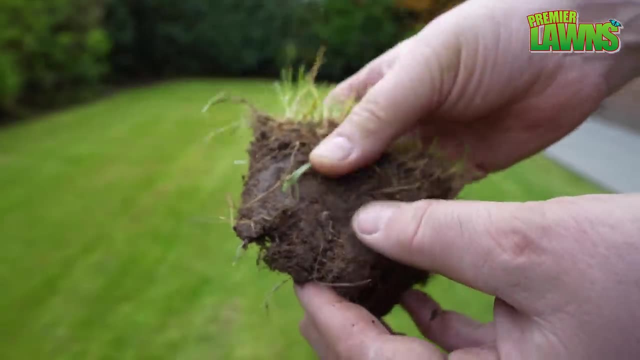 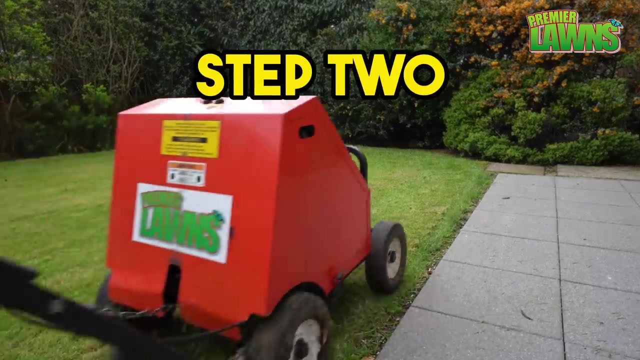 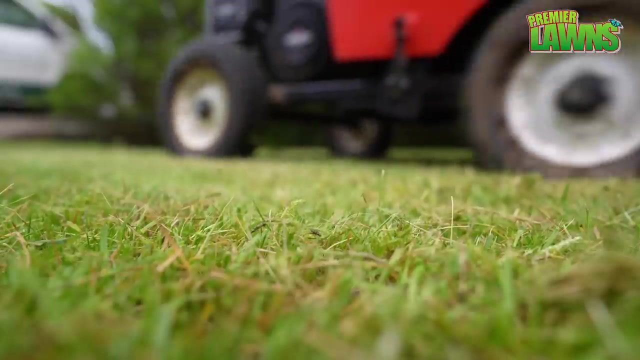 becomes a buyer there. but if we squeeze that together, you can just see it will have some worms and stuff in there, which is pretty good. I always like to see worms in the soil because that's going to indicate healthy soil. So that's the aerating done. so let's have a look just at some of the random. 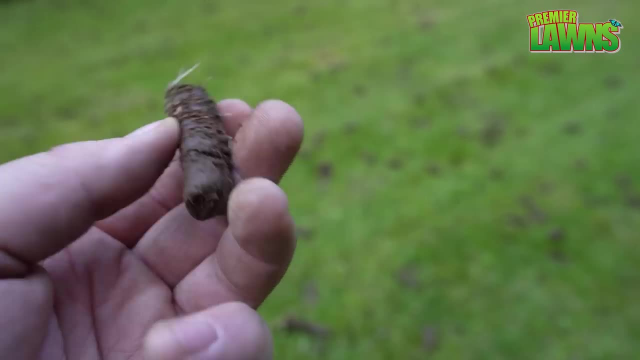 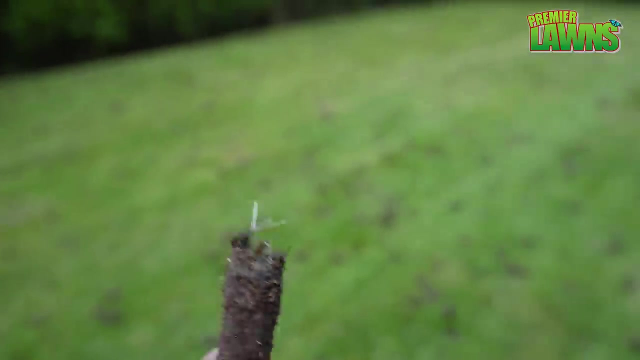 cores that were pulled out. You can see a wee bit of thatch on the top and a little bit of thatch on your lawn is good Whenever we have too much thatch, as we've previously explained, and it becomes a problem. these cores are the cores in this lawn. 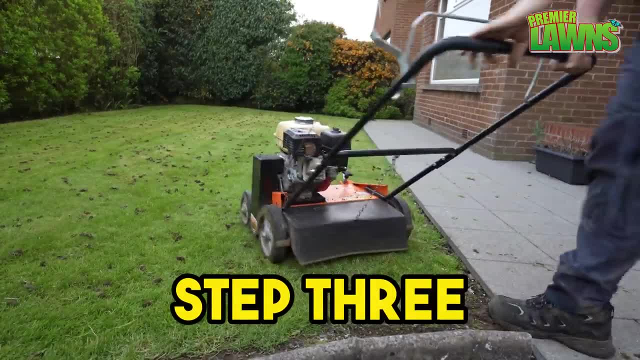 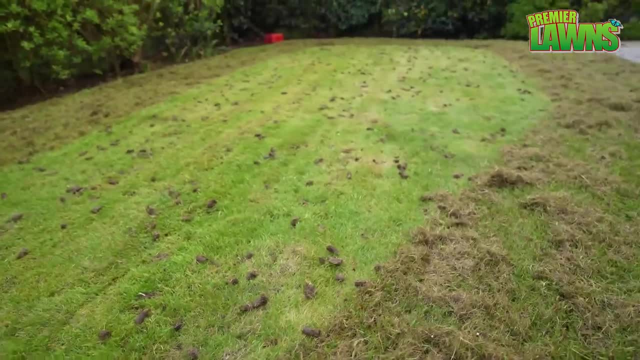 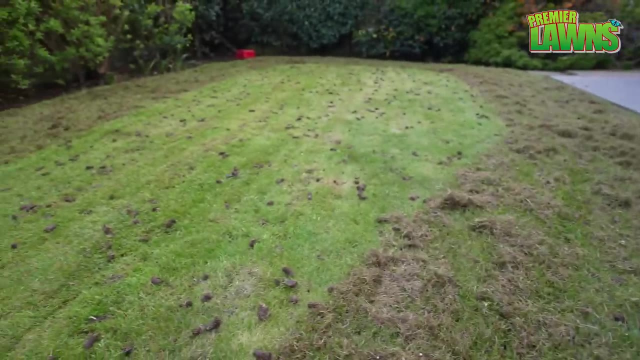 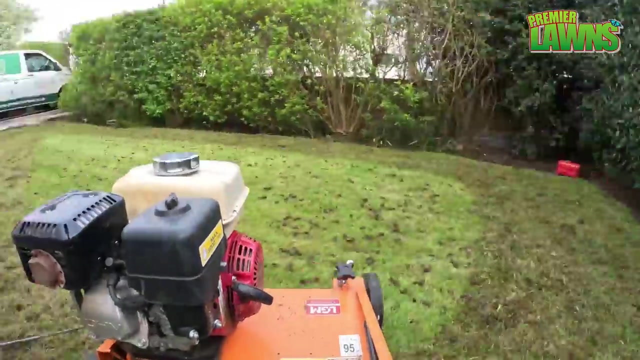 are fine. so just to have a quick look at it, you can see the usual affair. we have the moss and the thatch. this is just one pass. I am gonna do two passes over and I'm gonna go across to each other to take the most out. 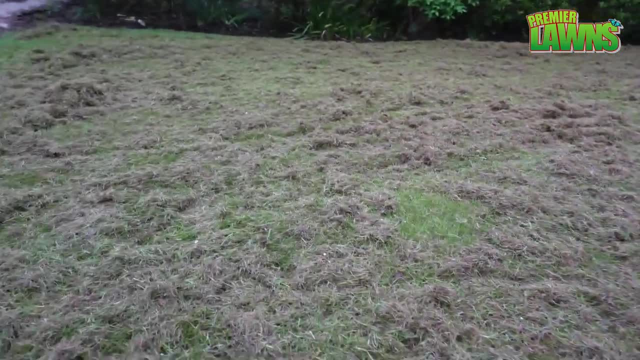 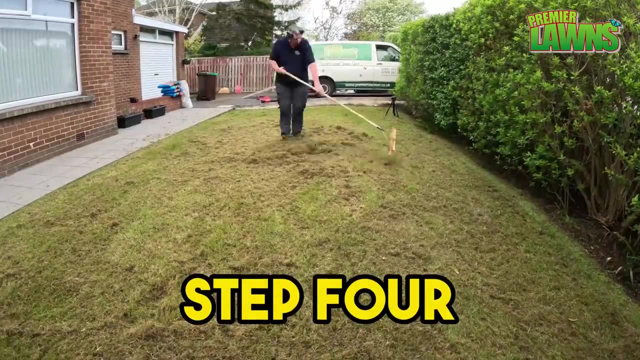 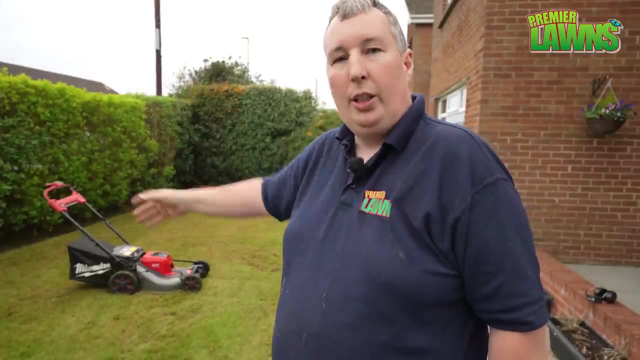 never fails to amaze me, whenever you scarify a lawn, just how much comes out with that small lawn. before we get on to the next bit, I'm going to take the lawnmower and run around the lawn. now I'm going to give a quick shout out to my sponsors, who are Milwaukee Tools UK. they're: 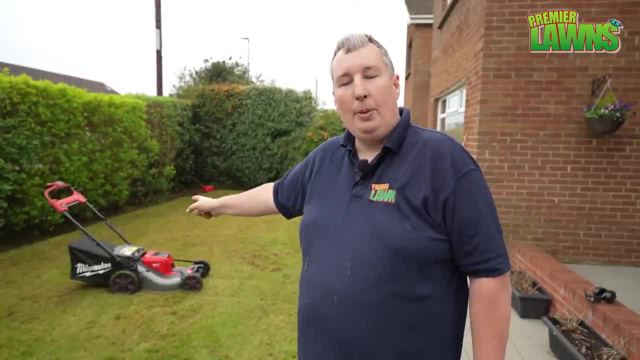 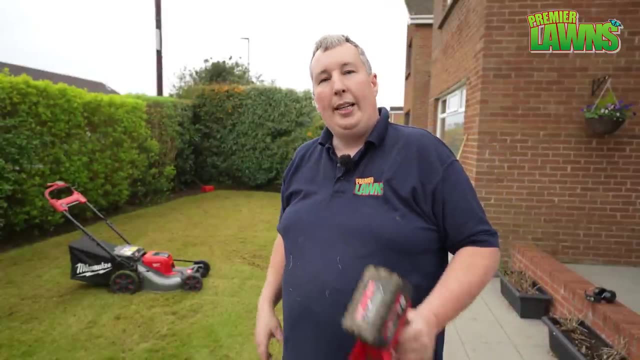 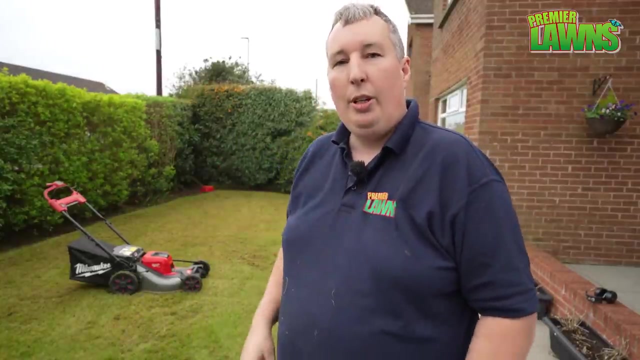 currently running a redemption offer that, if you pick up one of those Milwaukee lawnmowers from participating dealer- I'll leave a link down in the video description- you can redeem for a free blower, a free m18 hedge trimmer, the m12 hedge trimmer- this little blower has been fantastic and 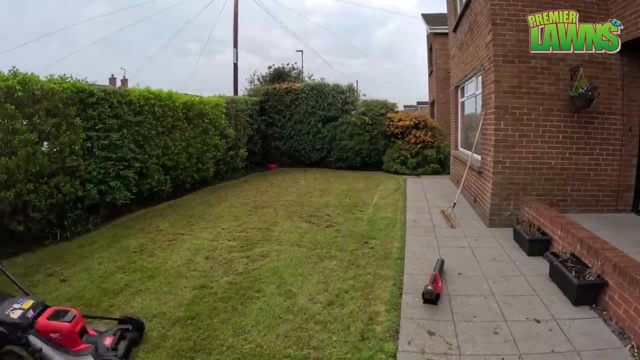 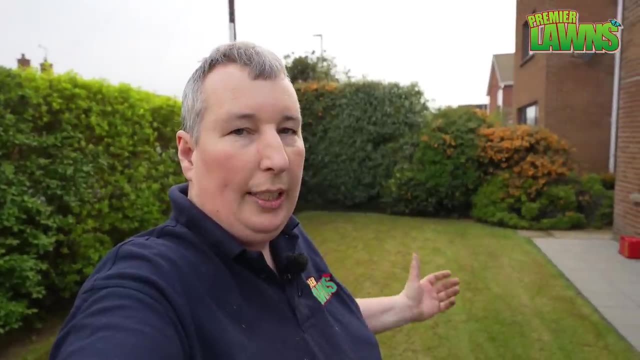 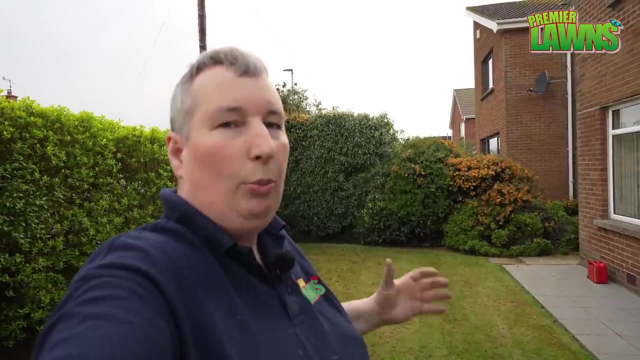 it is actually my most used tool out of all the tools that I own. my next task: now we've got the grass cut, we're going to get the compost roller out, seed it, mix some soil up in the compost roller, put it on, and that's going to put it on really well and I'm going to say I'm I'm really struggling. 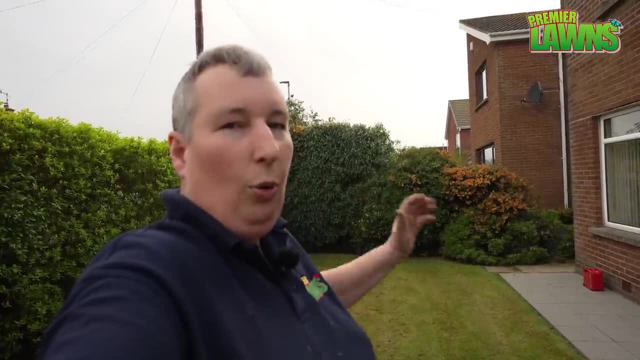 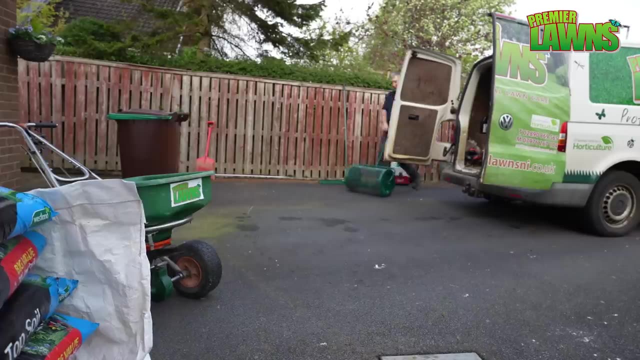 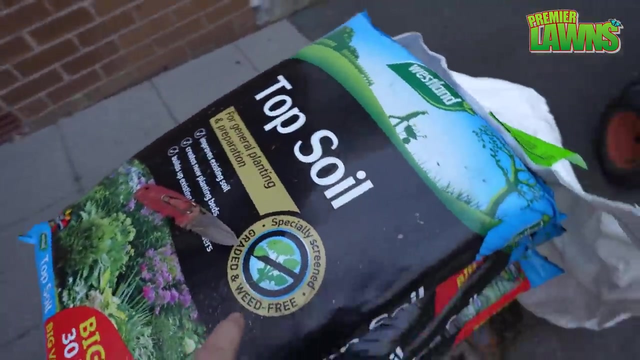 here because I'm filming this on a Friday evening after work. I don't want to be working in the dark. it's forecast to rain, so let's get on with it. so my next task is we're going to use the topsoil. I talk about this topsoil in a lot. 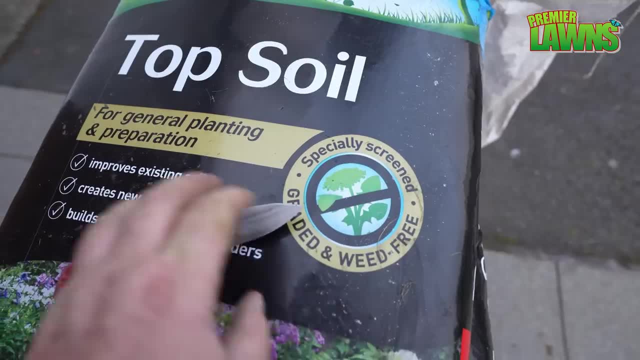 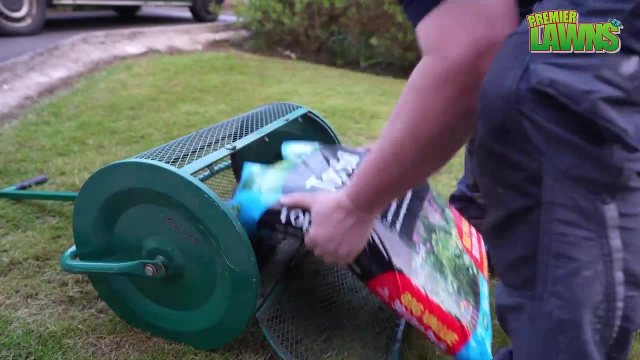 of my videos. the reason I use it is it's heat treated, it's weed free. so we'll put it in a so that we're throwing a bit of soil into that, we'll throw some seed onto it and then we'll put it onto the lawn. so anytime you're going to the garden center to buy these here, 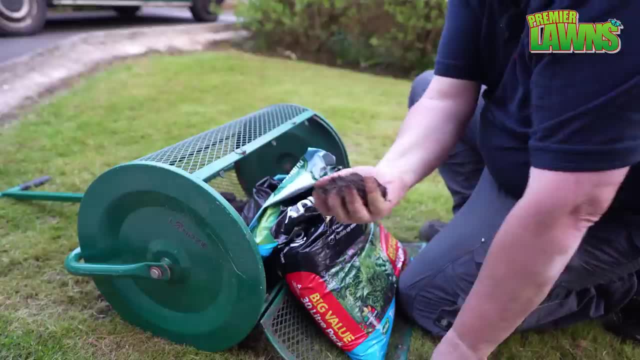 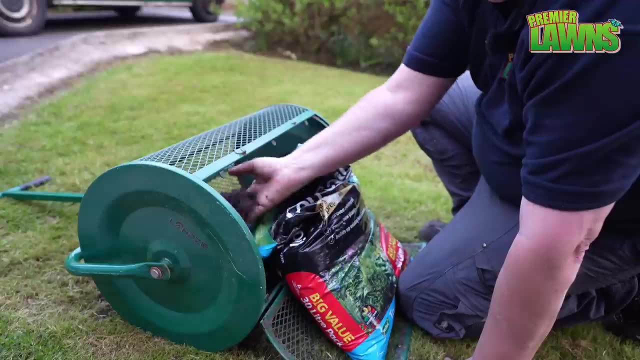 bags always check to make sure they're dry that stuff. there's still a bit dumped, a bit dumpier than I would like, but the stuff at the top was really dry, the stuff at the top was really wet. so so my advice if you're going to the garden center to pick this stuff up. 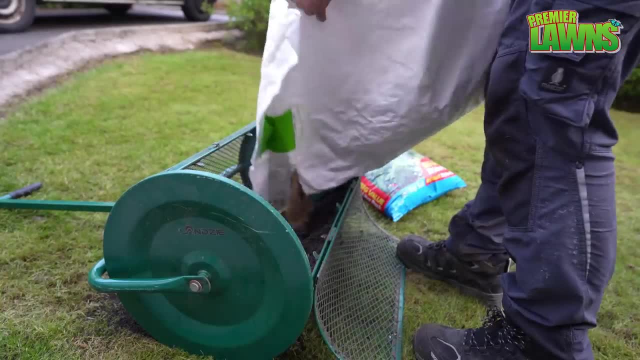 always take it up from below the bottom of the stack. so for grass seed today, that's what we're going to use the bottom of this bag for. so now, just someгиou pots forgotten. my little izabara saying so. we're going to add some. we're going to add other Dana hi to the. 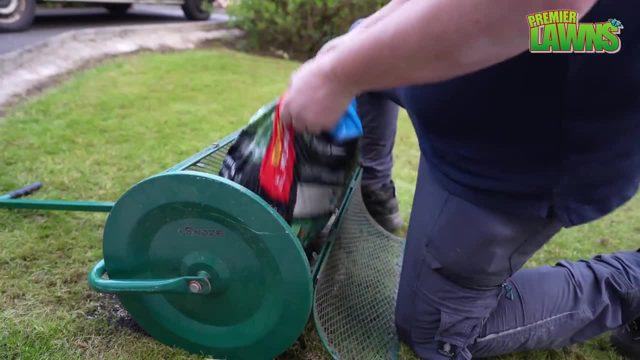 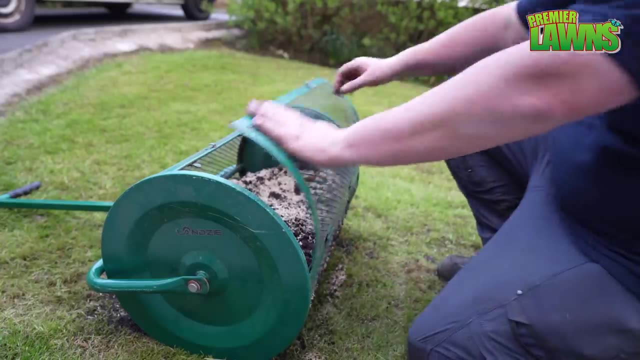 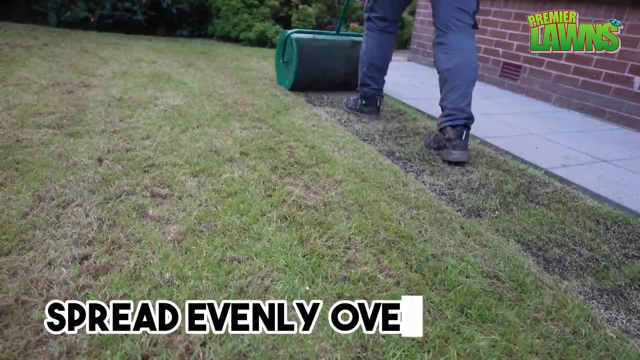 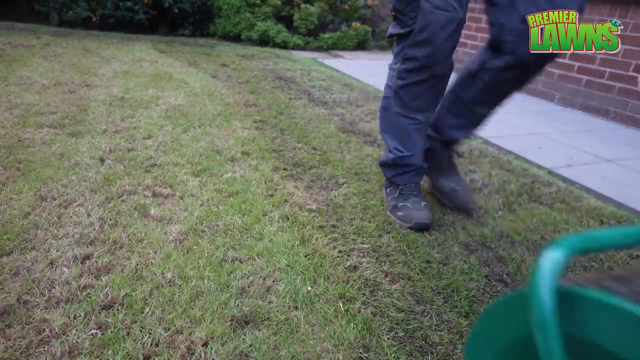 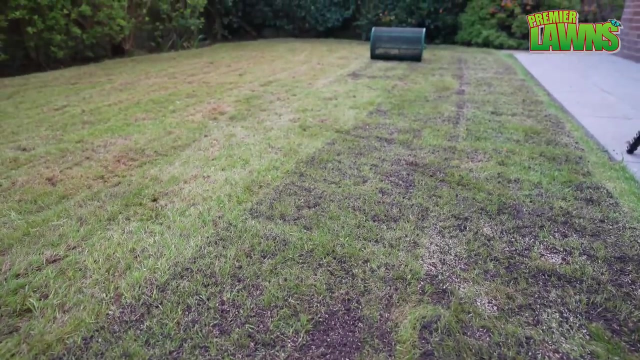 we're going for a rye fescue mix. We'll have that in now. let's put in a bit more seed. All I'm going to say is the soil's a little bit dumber than what I would like. It is coming out okay, but I'm finding I'm having to do a couple of passes. 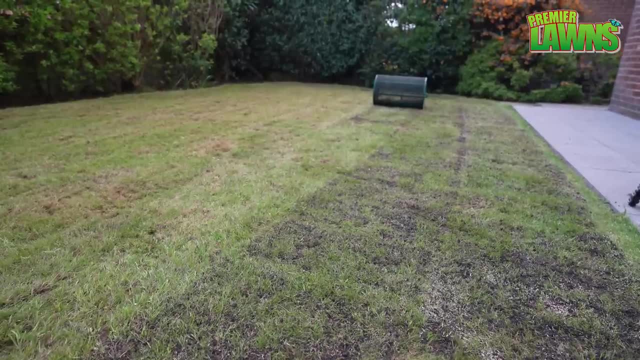 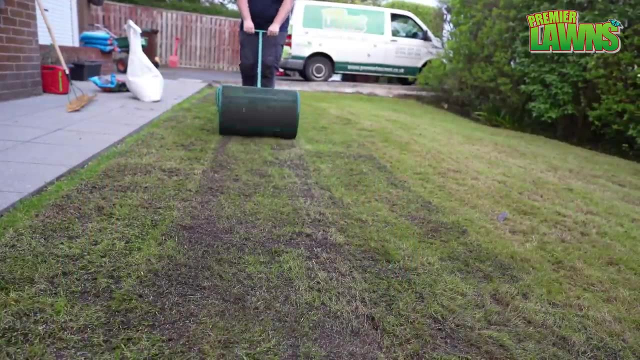 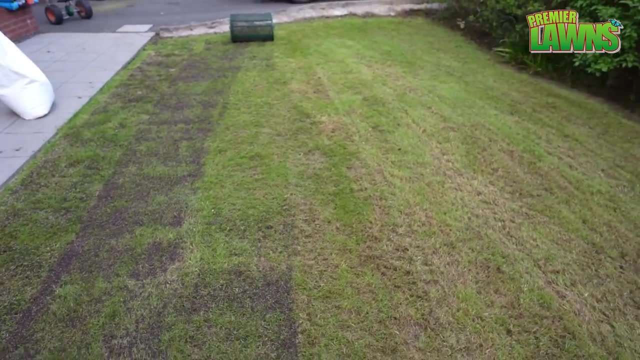 If the soil is dry, you do one pass and it's over. and it's brilliant, it's really really quick. Two passes definitely isn't the end of the world. a lot, lot easier than using a shovel. So that's one bag so far. I have four bags with me, so we're gonna go one, two, three, four. 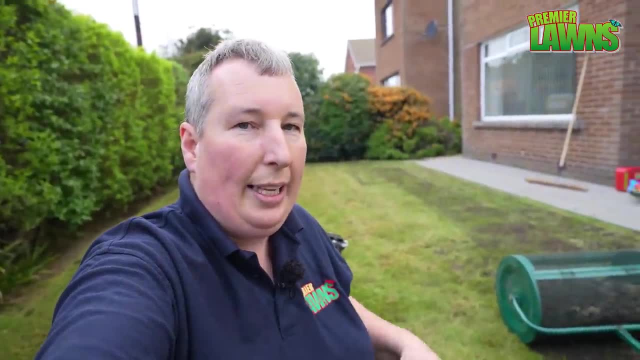 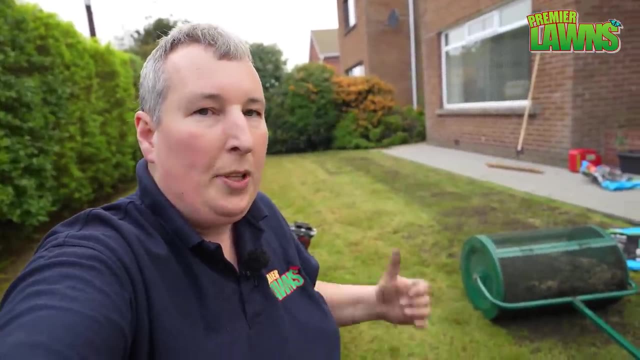 Just about with four bags. Today we're seeding with the rye and the fescue. Rye is a good hardwiring grass seed. there's a lot of rye already in this lawn. We're going for some fescue as well. there's some fescue here as well. 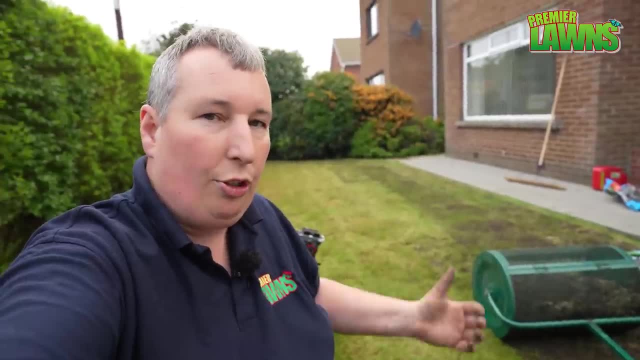 We've got the shade. the fescue is going to do well in the shade. If you just go with 100% rye, then it's going to thin out a lot in the winter and we don't want that. We want a nice, even lawn the whole year round. that's the benefit. 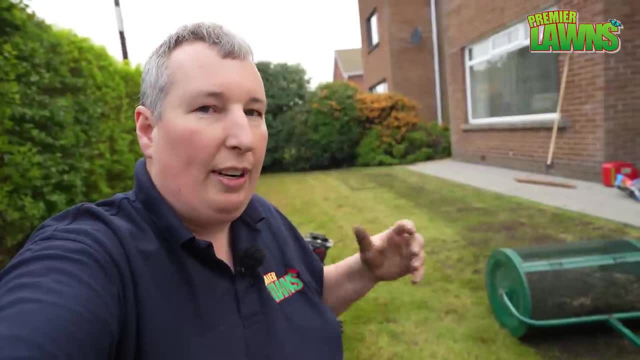 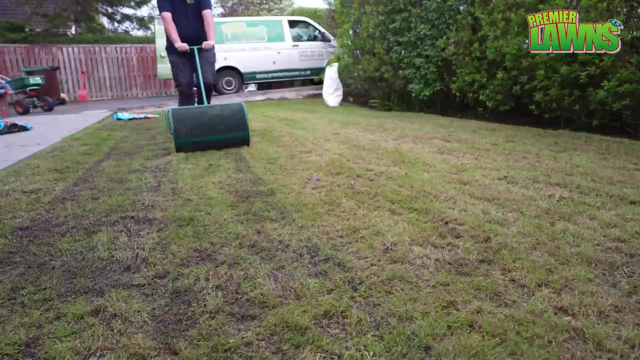 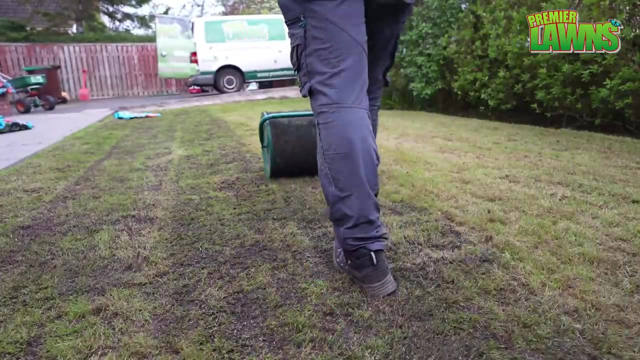 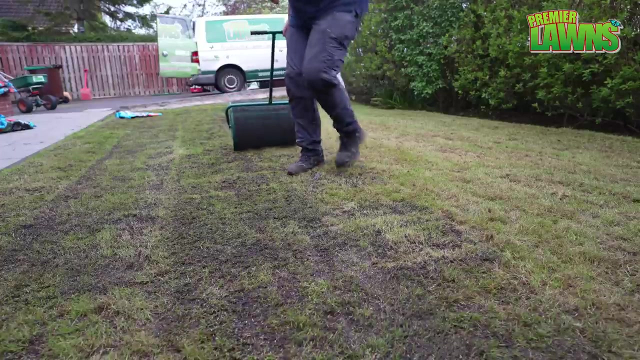 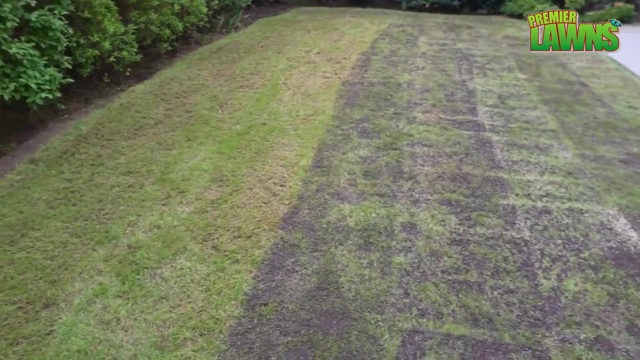 of using a couple of different grass seeds. I suppose the minute seems very fashionable just to use 100% rye. the problem with that is it thins out in the winter, Coming out a wee bit better now. So there we go. we're halfway. two bags down, two to go. 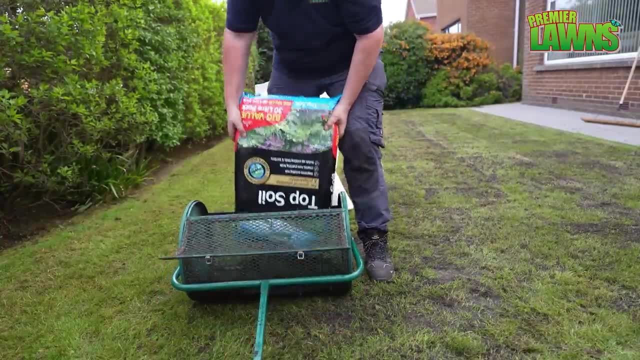 Just going to say last time, the first time, I put in too much seed. last time, I think, I put in a good amount, so we're going to do something similar this time. So put in about three quarters of the bag and then hand ball a lot in. 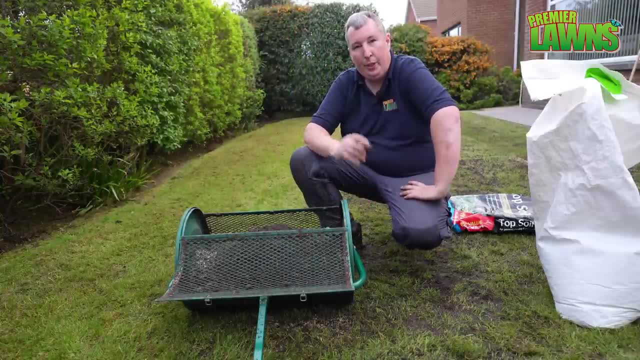 A lot of people are always asking me: how much seed do you put in? What I say is: there's no hard and fast rules, just play about with it, put some in, mix it up, put it out, see how you go. 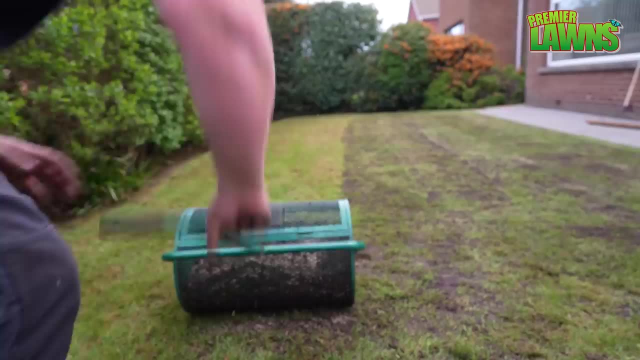 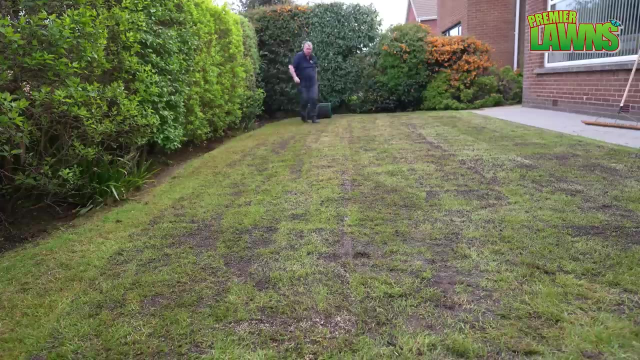 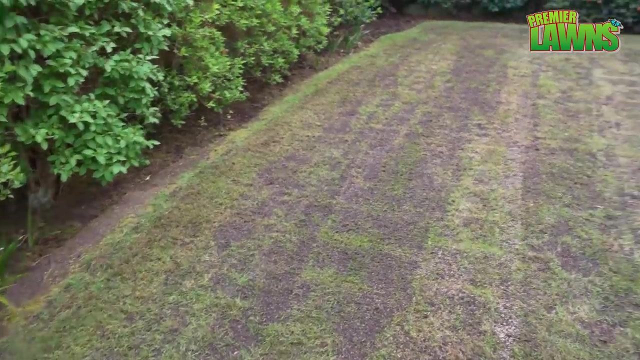 You can always put on a bit more and you'll just learn by experience. Have a bit of fun. So in the end I only used the three bags. the last bag that I used wasn't as dump. Now let's go and have a look and see what we've got in it. 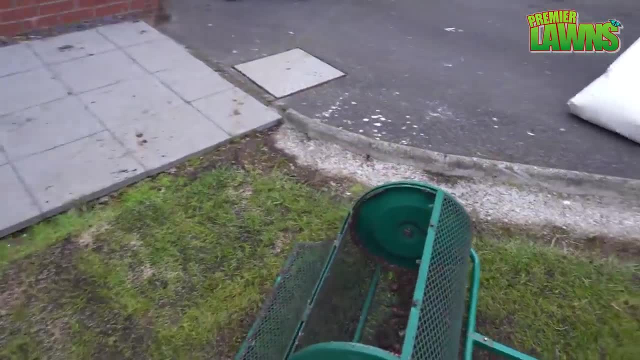 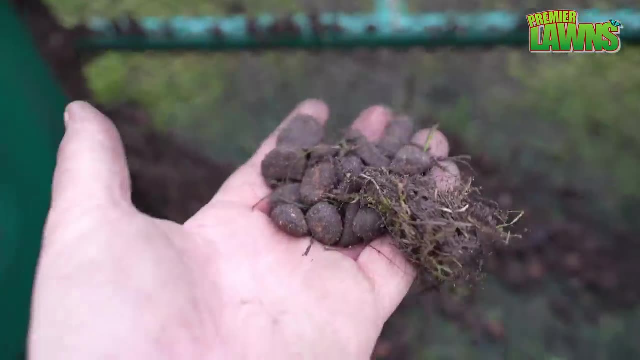 Just to see all the stuff that stops from landing on your lawn. Quite a few stones through this. If I was putting this on with a shovel then I'd have to rake all these stones off it and it might make a lot of noise. 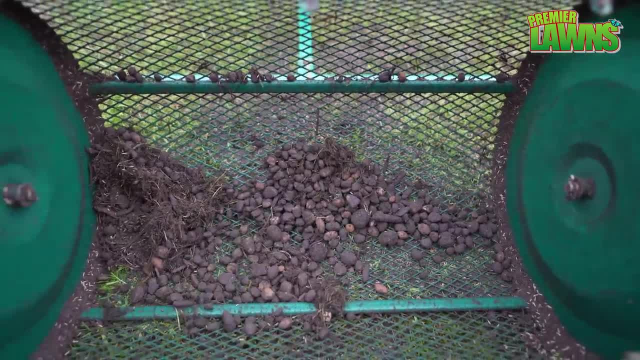 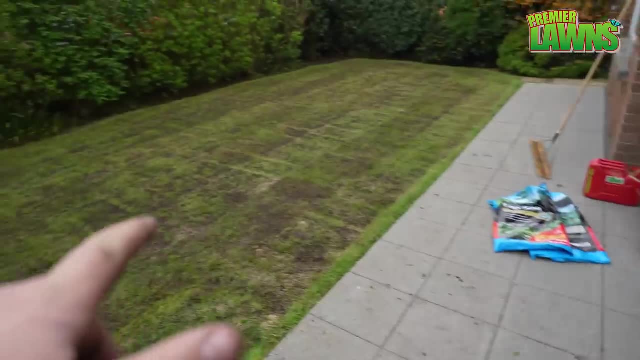 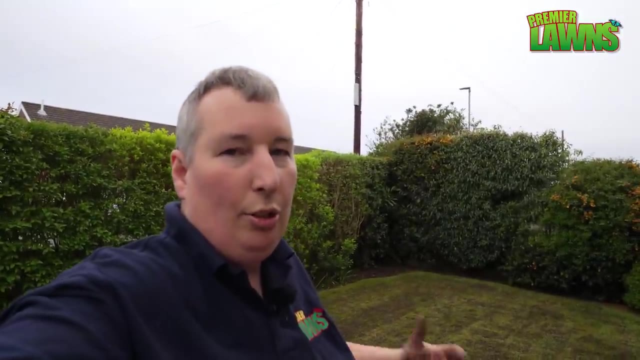 Like I said, if we were put that on with the shovel, we would have used a lot more and it wouldn't have been as even as it currently is. Today, I'm not going to be using the mat, I'm actually just going to be using the laminate. 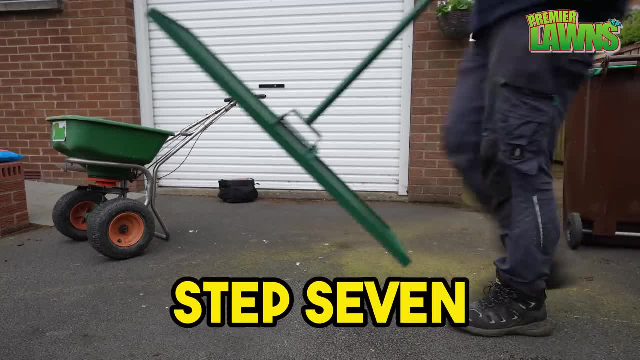 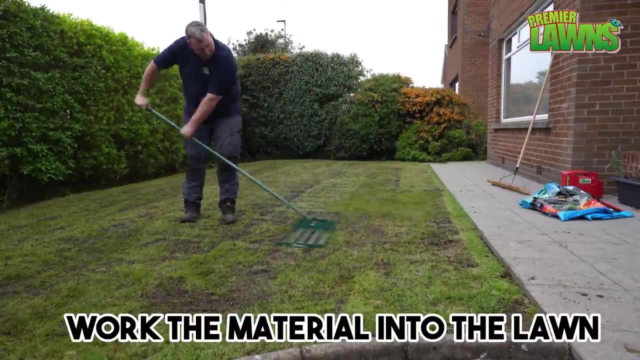 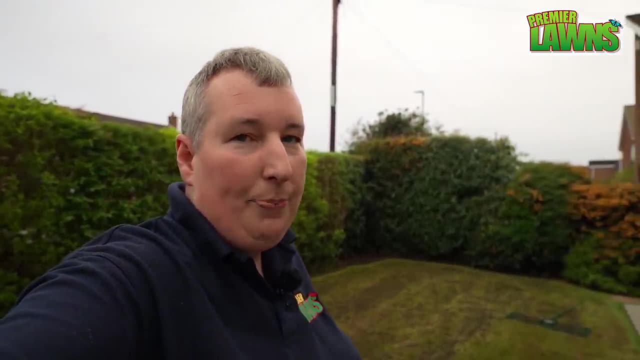 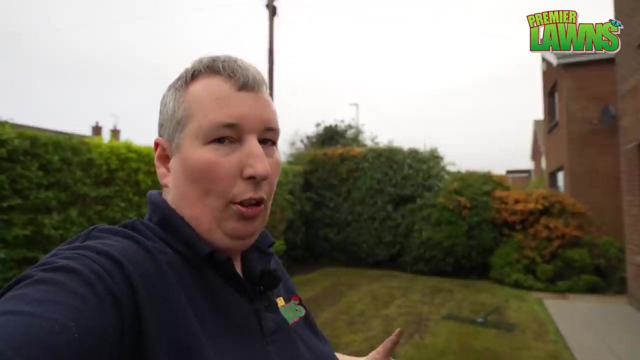 I forgot to put the mat in the van. Now I'm breaking one of my golden rules here. I always say that you should leave it to dry. Unfortunately, I don't have that luxury, But the minute it's trying to rain, trying to rain, and it's getting very late and it's going to start getting dark soon. 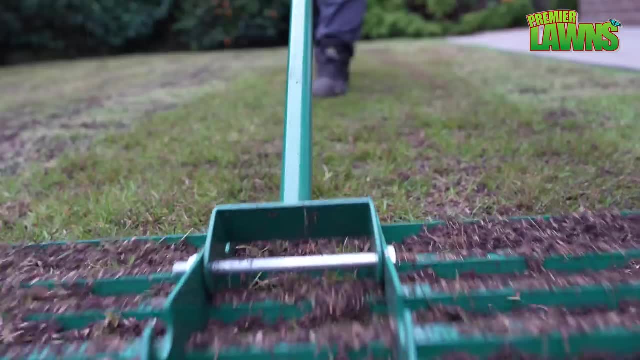 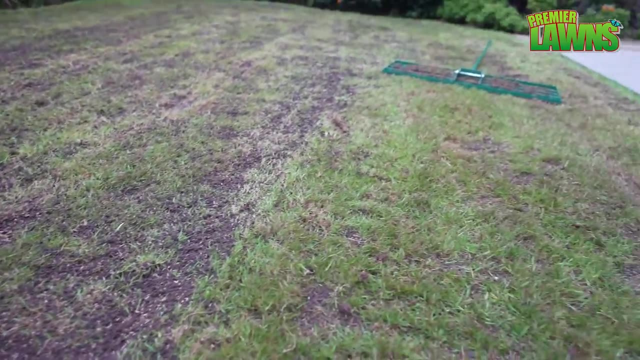 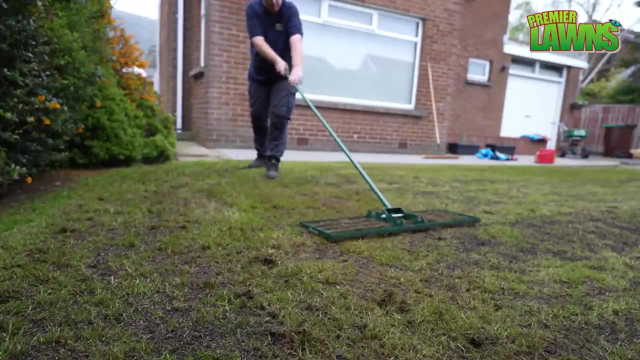 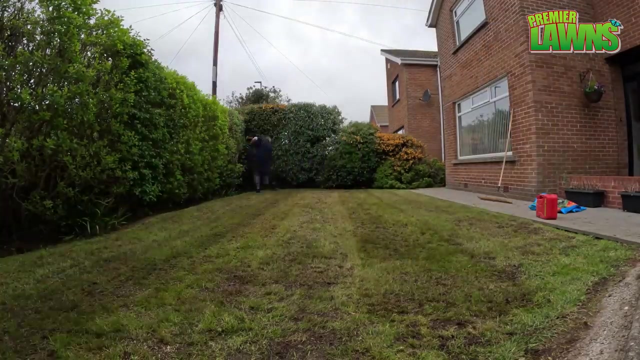 So I'm just going to have to crack on with it. So there's the bit that we've soiled, And then just one or two passes with the laminate has matted it in. really well, That's us, we've got it matted in. 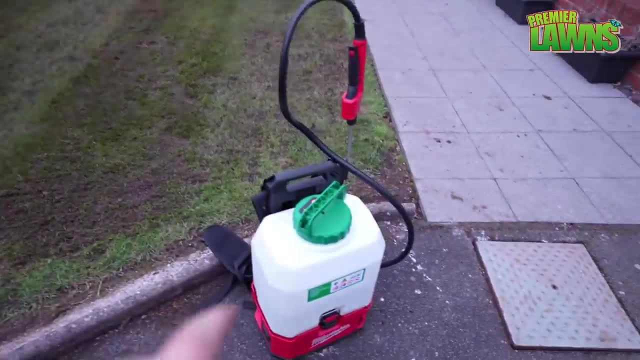 It is starting to get very dark, so we have to be quick. My next task I'm going to do the seaweed. I went to Donegal during the winter to find out all about seaweed and why seaweed is so good for your lawn. 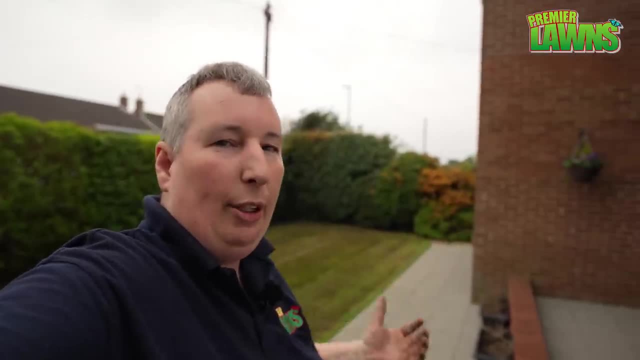 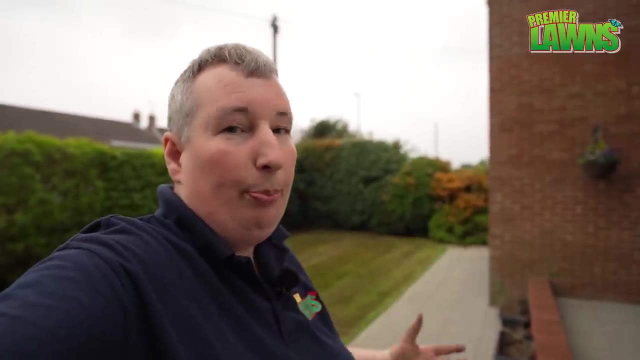 If you want to find out more about seaweed, I'm going to leave a link down in the video description. That video was really. it blew my mind going to film it And I'm going to say that if you watch it, you'll definitely learn something from it, if you pay attention to it.